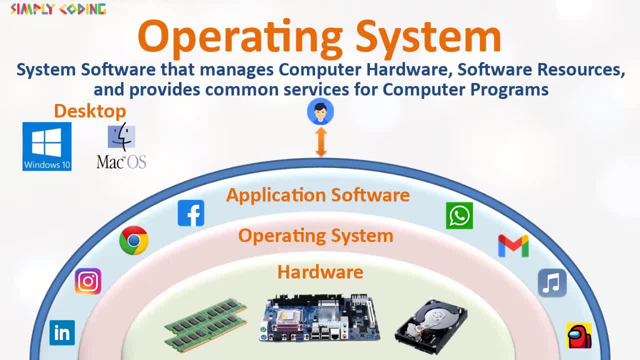 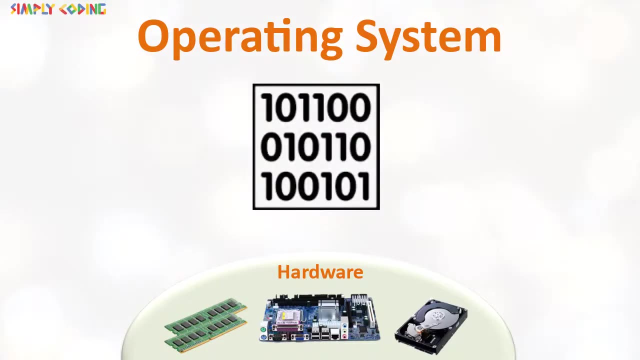 Examples of operating system are Microsoft, Windows, Apple's Mac OS, Linux for computers, Android, Apple, iOS, Symbian for mobile phones. Why do we need operating system? This is because computers can understand language of only ones and zeros, which is called as machine language. 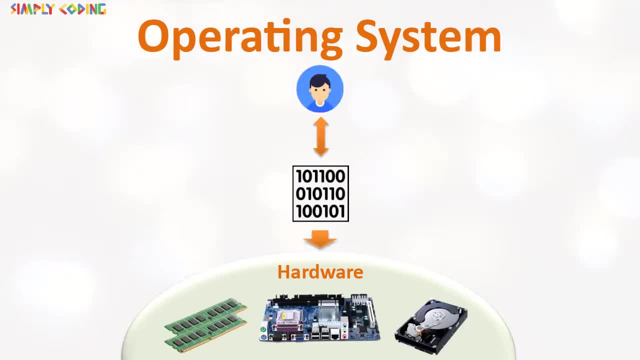 So initially the computers were given instructions in ones and zeros by punching on paper cards To make our work easier. slowly, features were added for it to understand assembly code, error detection and handling, allocating resources, managing memory, etc. So its advantage was that it effectively allowed you to 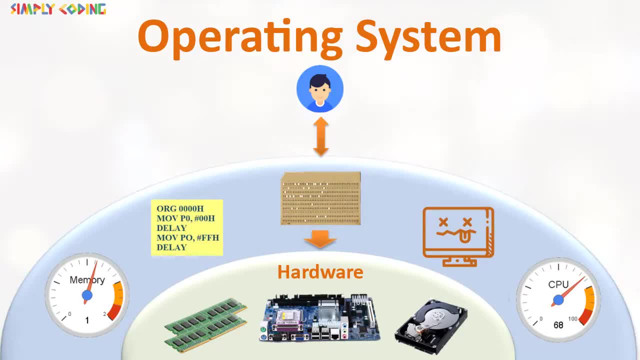 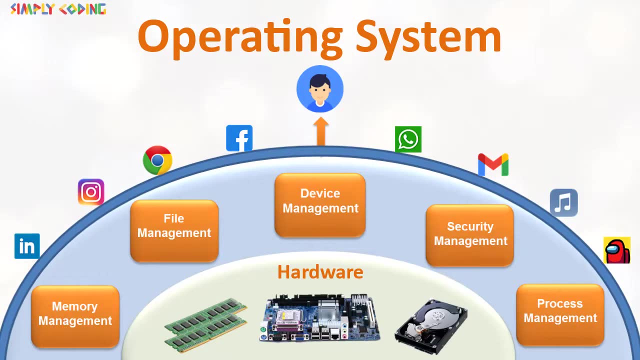 hide the detail of hardware by creating an abstraction and making the computer easy to use with rich graphical user interface. These features are clapped into various functions which are offered by a modern day operating system. Let's look into each of them in detail. First is 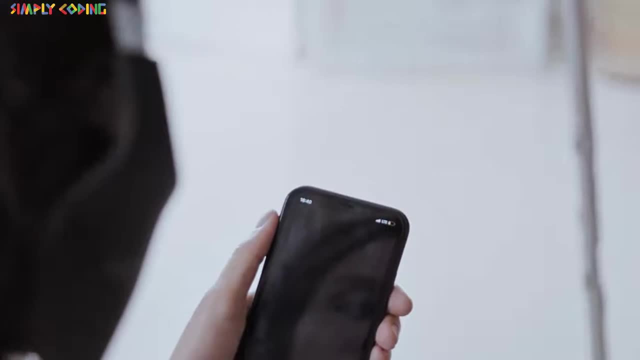 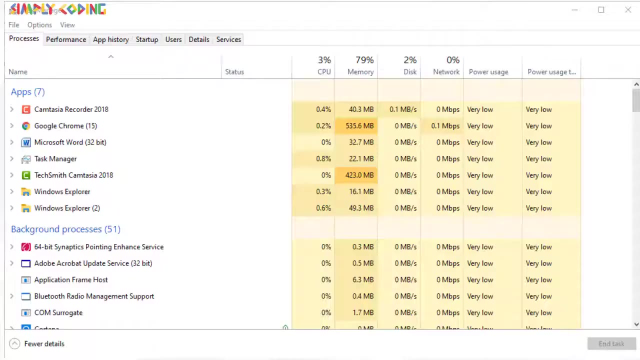 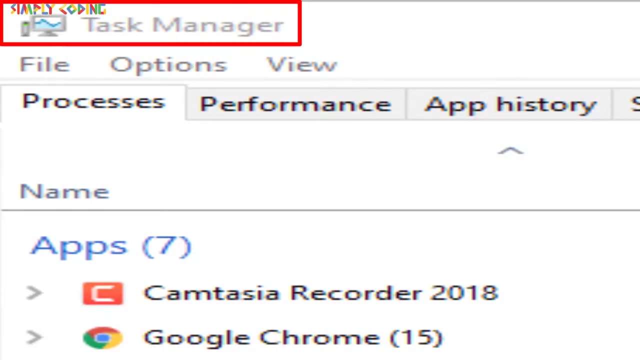 process management. We use computer to do multiple things simultaneously, Like you could be listening to music while browsing on a social media app. In Windows OS, you can view the processes which are running by opening the task window. A task in execution is called as process. 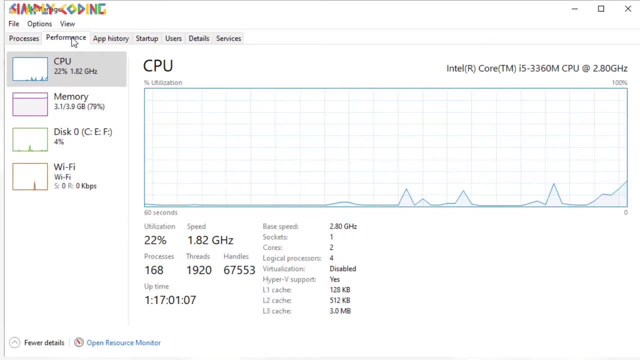 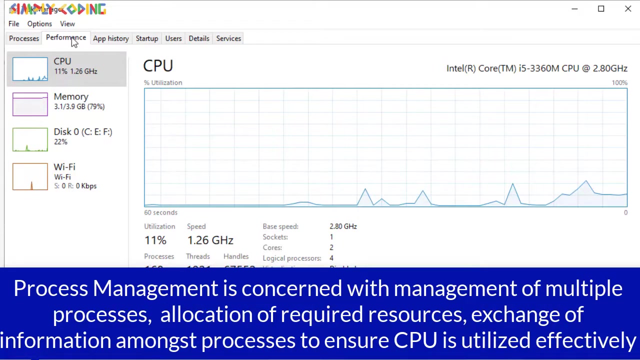 One of the key functions of OS is to prepare, schedule, control, run and monitor jobs on CPU so that it is effectively utilized. So process management is concerned with management of multiple processes, allocation of required resources and exchange of information among processes to ensure CPU is utilized. 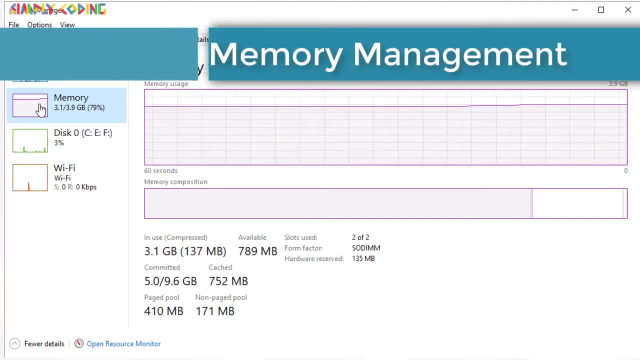 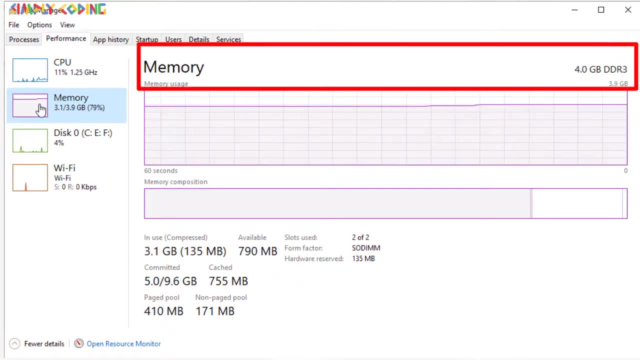 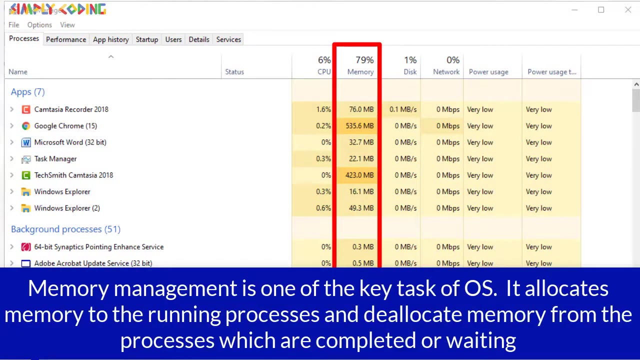 effectively. Next is memory management. All of the tasks we execute on the computer require memory. The primary memory, or RAM, is limited. One of the key tasks of OS is allocate memory to the running processes and de-allocate memory from processes which are completed or 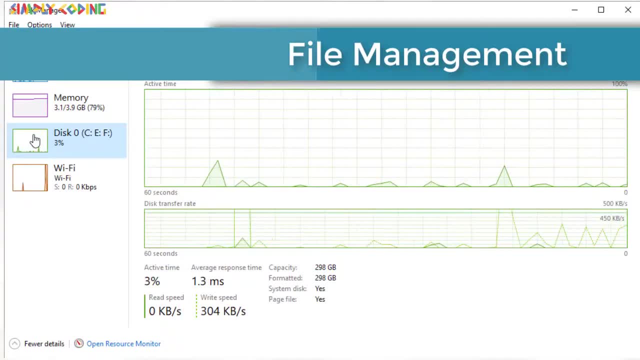 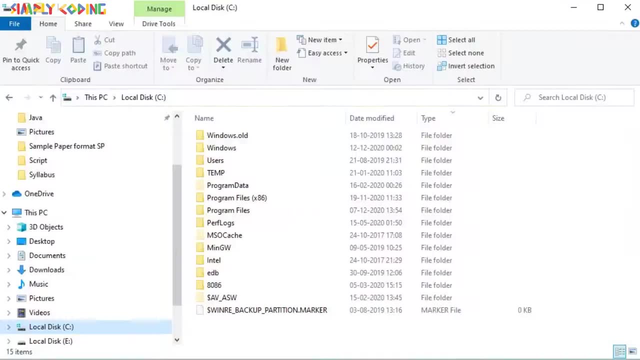 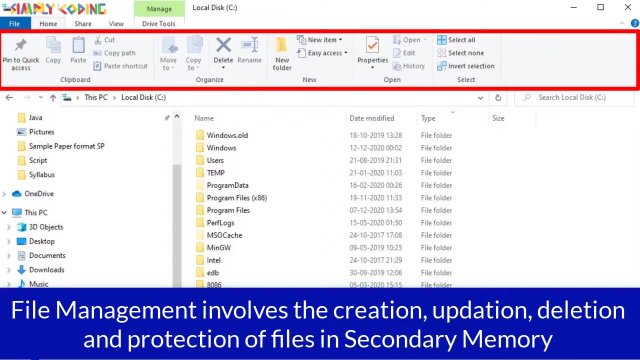 waiting. Next is file management. Many processes require the use of secondary memory, like storing or retrieving information from hard disk. File management involves the creation, updation, deletion and protection of these files in the secondary memory, So where memory management is managing primary. 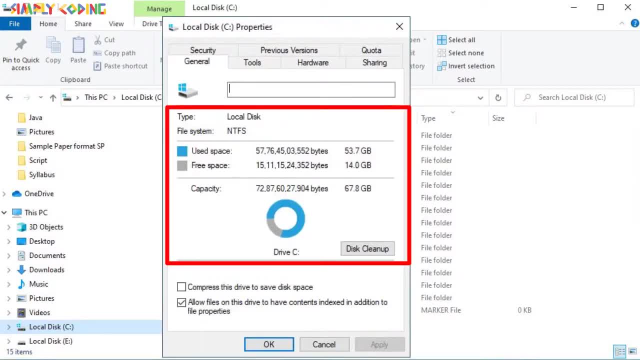 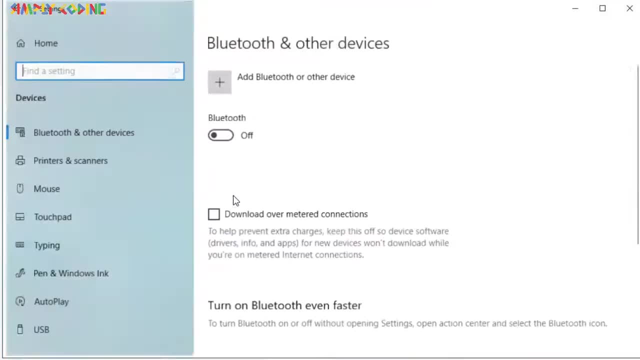 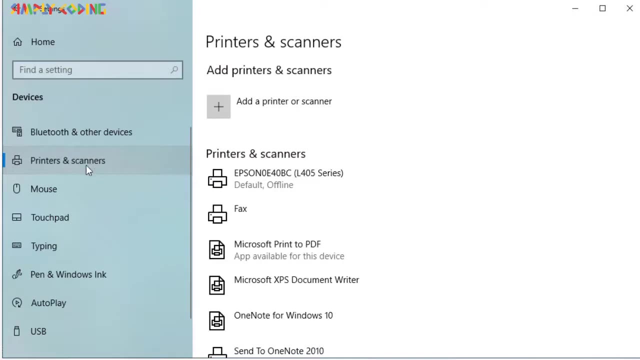 memory. file management is all about proper management of secondary memory. Next is device management. We use so many input and output devices like headphones, speakers, printers, etc. It is the function of operating system to ensure it interacts with device drivers or related. 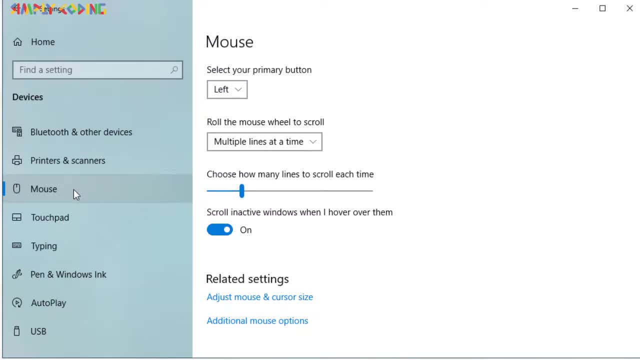 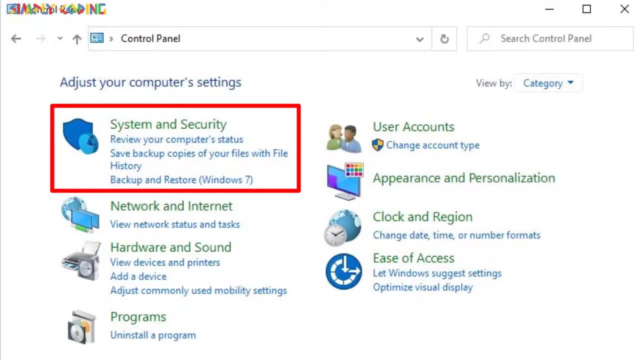 software to configure and operate the devices as per user requirement. Other than these basic features, OS is also responsible for security by means of password and restricted access, networking and providing a user friendly interface. Based upon type of interface provided, operating system can be divided into. 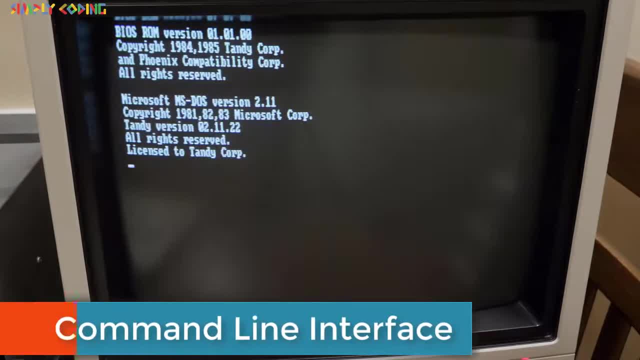 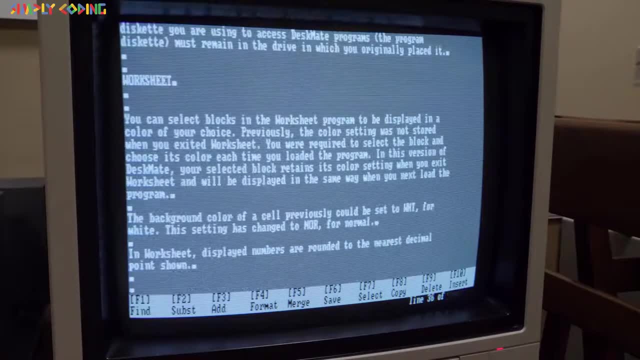 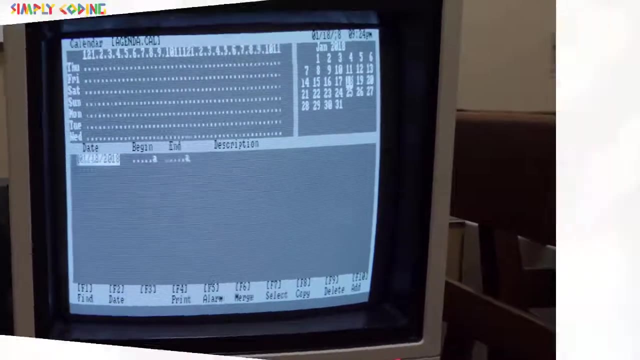 multiple types. Initial version of OS only had command line interface. This was before mouse came into picture and user had to remember and enter the commands on the screen. Example: MS-DOS operating system developed by Microsoft. Then came in OS with graphical user interface or GUI. 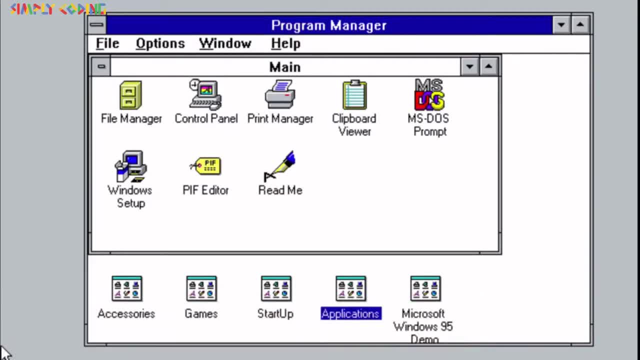 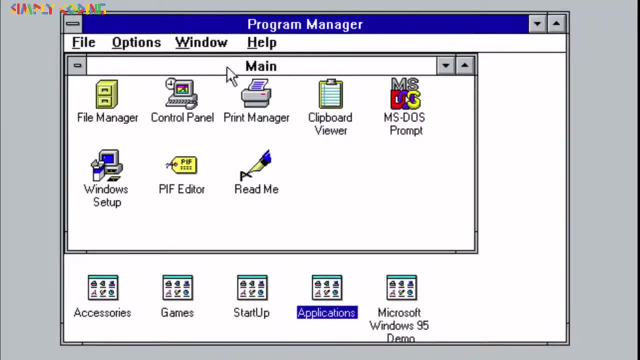 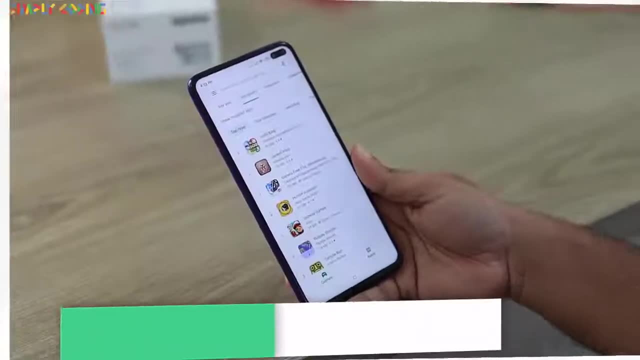 which lets user run programs or give instructions to the computer in form of icons, menus and other visual options. These made interactions with computer easier and computer could be operated with a mouse. Nowadays, smartphones, tablets and PCs allow user to interact with the system simply. 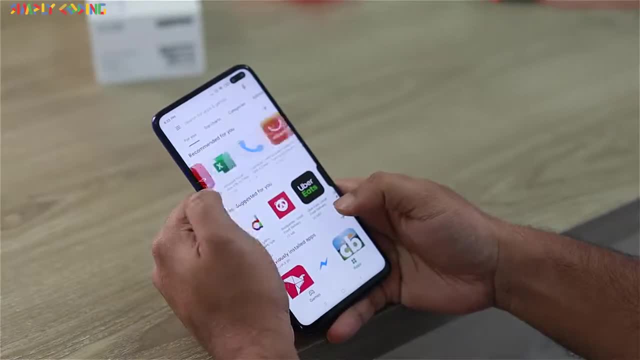 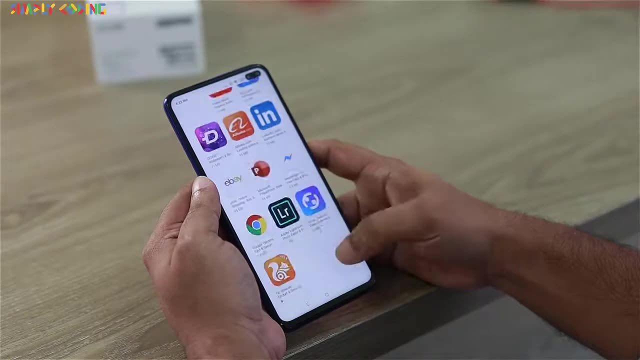 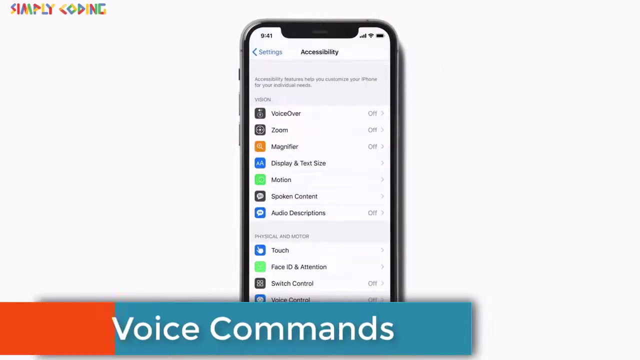 by using the touch input. Many operating systems have integrated the touch screen technology to allow user to provide input via a touch screen, like latest version of Windows, Android, iOS, etc. To address needs of people with special needs. latest OS versions also provide voice based controls.